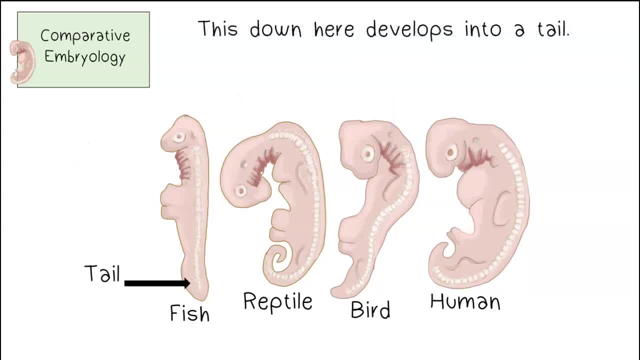 humans. This down here develops into a tail In the earliest stages of development. tails are found in all vertebrate species, even if they don't grow and develop to actually have a tail. The similarities found in the embryos of species that grow up to be very different are evidence. 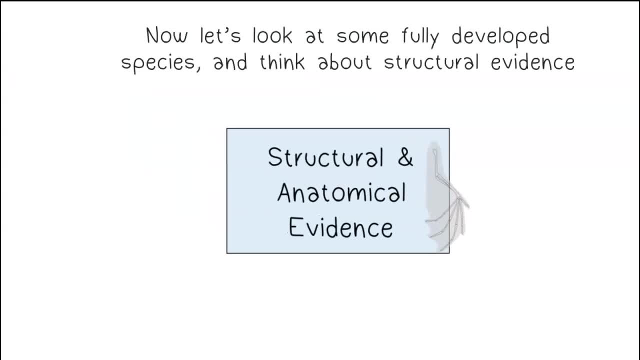 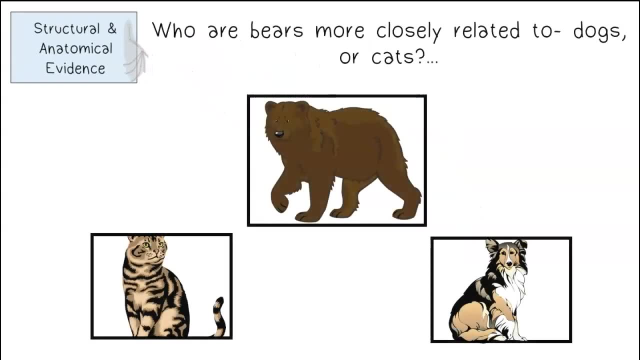 of common ancestry. Now let's look at some fully developed species and think about structural evidence. Who are bears more closely related to dogs or cats? Well, if I had to take a guess, I would think about who bears are more similar to. 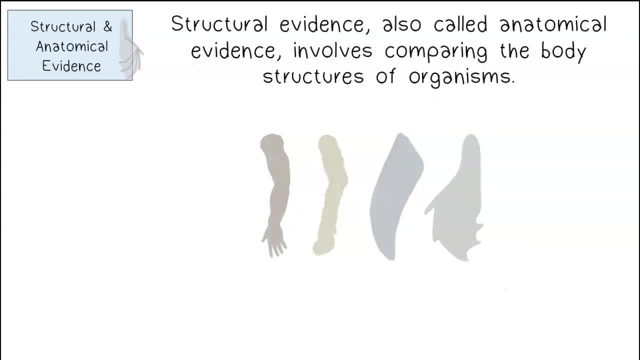 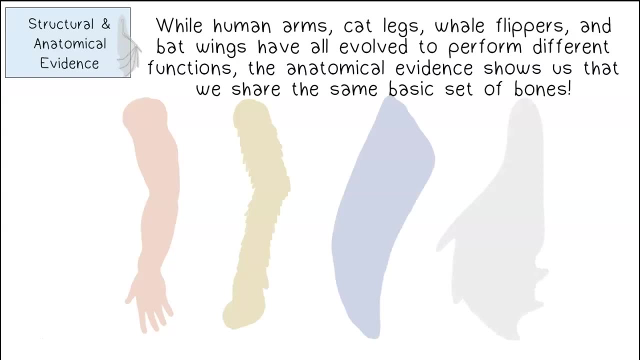 Structural evidence, also called anatomical evidence, involves comparing the body structures of organisms. This could include comparing teeth, bones or organs, For example. while human arms, cat legs, whale flippers and bat wings have all evolved to perform different functions, the anatomical evidence shows us that we share the same basic. 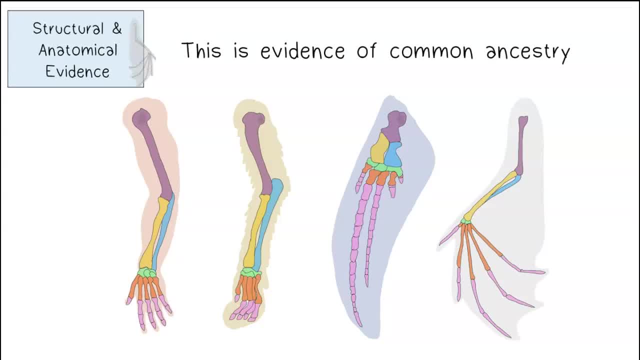 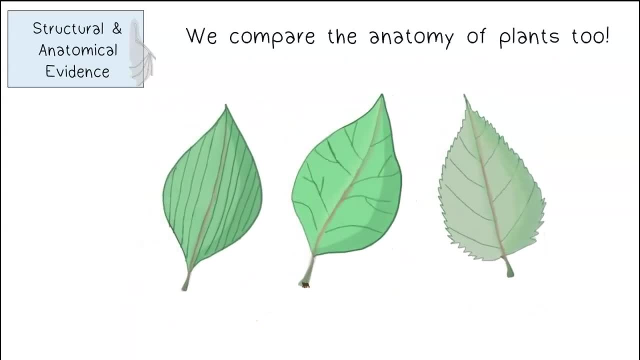 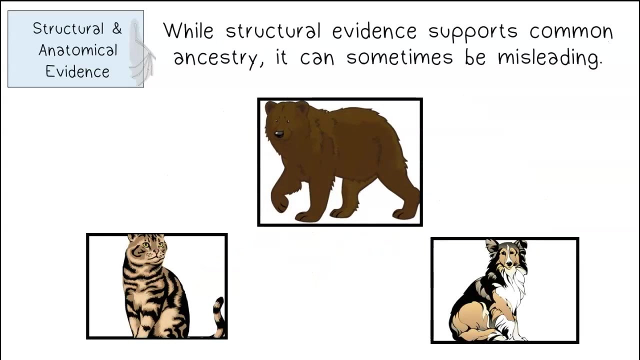 set of bones. This is evidence of common ancestry, but it's not just limited to species that have bones. We compare the anatomy of plants, too. While structural evidence supports common ancestry, it can sometimes be misleading. Did you know that the closest living relative of a bear is actually a seal? 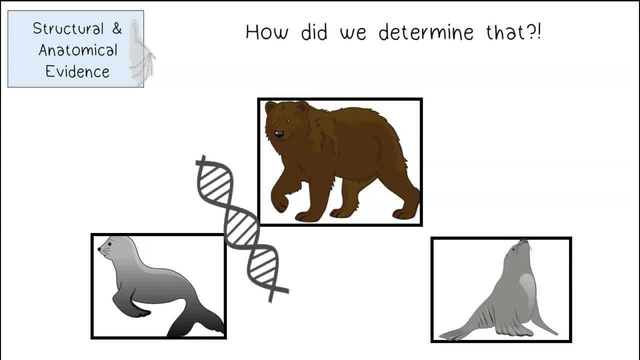 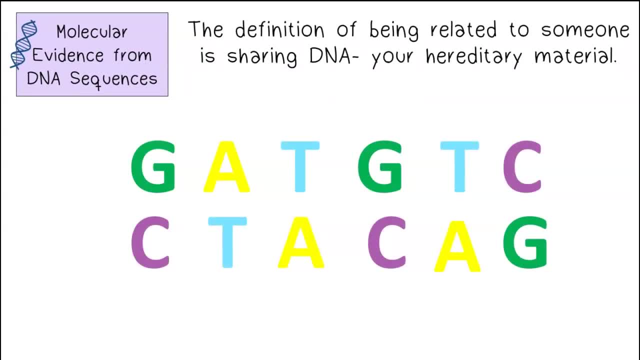 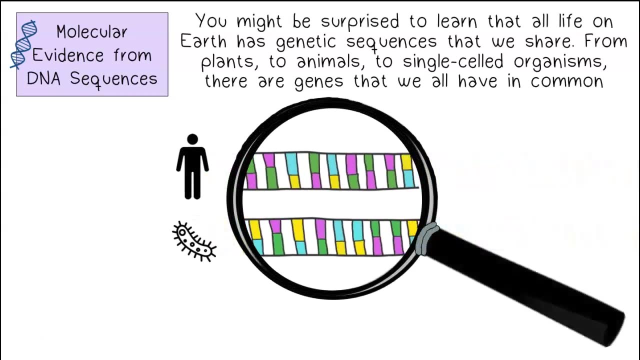 How did we determine that? Well, through DNA evidence. The definition of being related to someone is sharing DNA, Your hereditary material. You might be surprised to learn that all life on Earth has genetic sequences that we share, From plants to animals to single-celled organisms. there are genes that we all have. 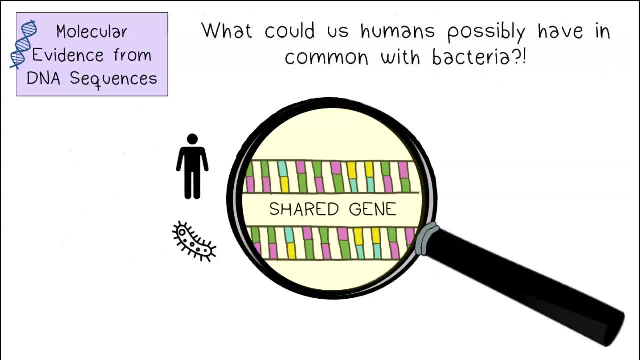 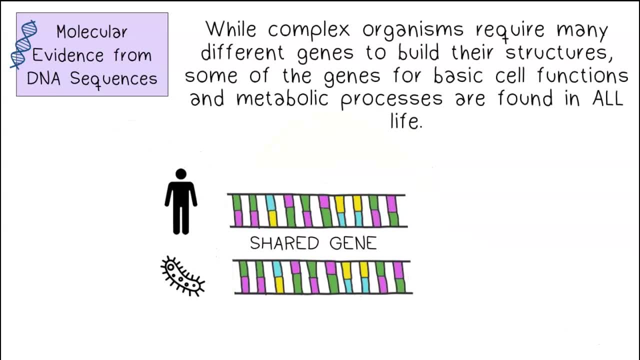 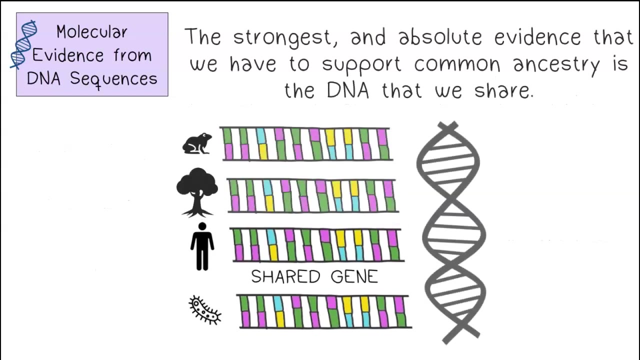 in common? What could us humans possibly have in common with bacteria? While complex organisms require many different genes to build their structures, their genetic processes are found in all life. Some of the genes for basic cell functions and metabolic processes are found in all life.